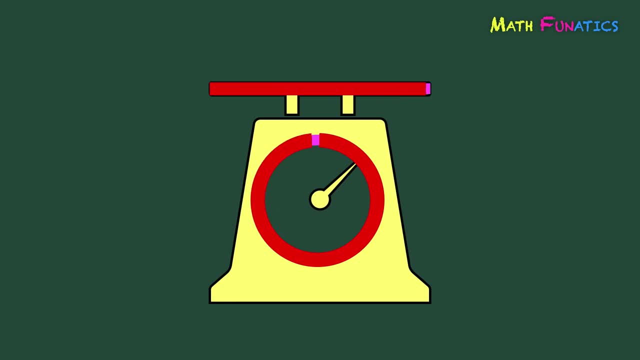 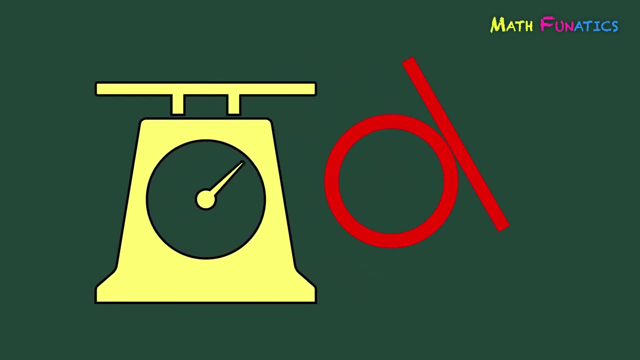 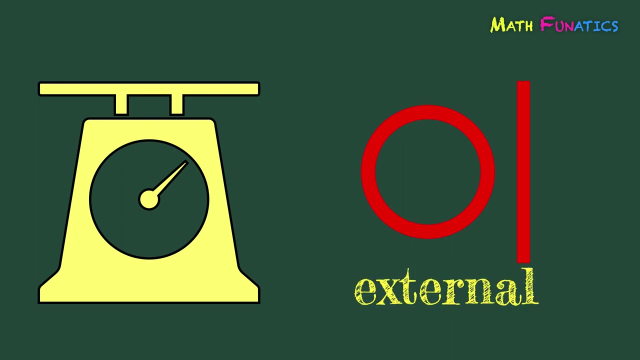 In the first figure, the circle and the straight line are apart from each other Or they have a certain distance in between them. This case, when a line is outside and does not intersect a circle, is called external. The external line does not have a common point with the circumference of a circle. 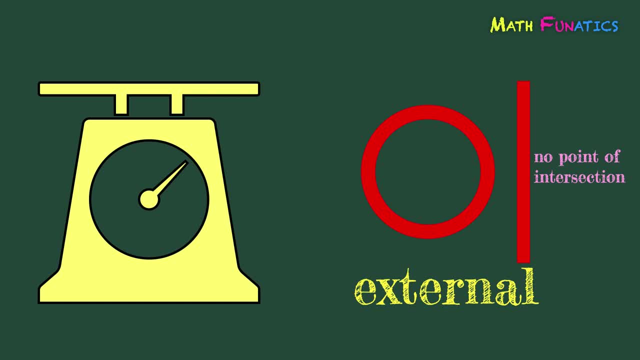 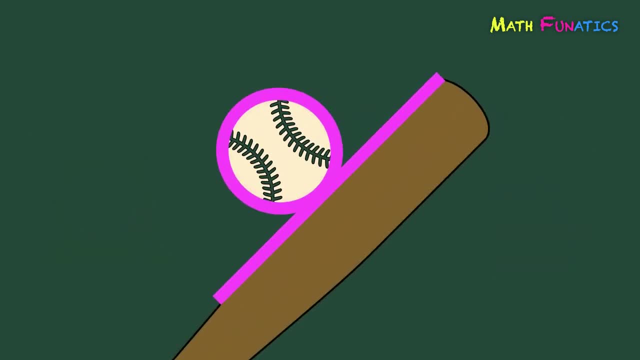 So there is no point of intersection. This time let's analyze the baseball and the baseball bat. In this figure, the baseball, which is circular in shape, is touching the straight edge of the bat at a certain point. This case, when a line and a circle meet, is called tangent. 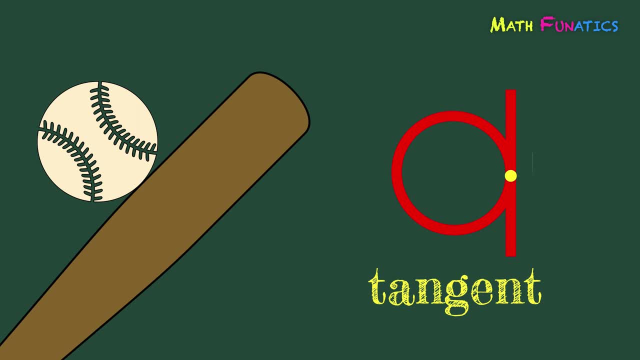 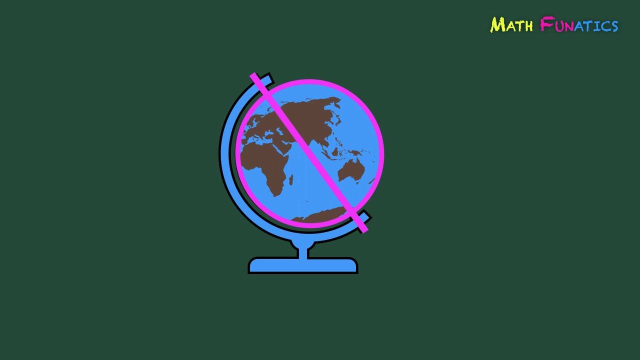 The straight line and the circle have one common point or point of intersection, And this point of intersection of the tangent line with the circle is called point of tangency. Finally, let's take a closer look at this globe. In this figure, the axis which is a straight line passes through the globe that is circular in shape. 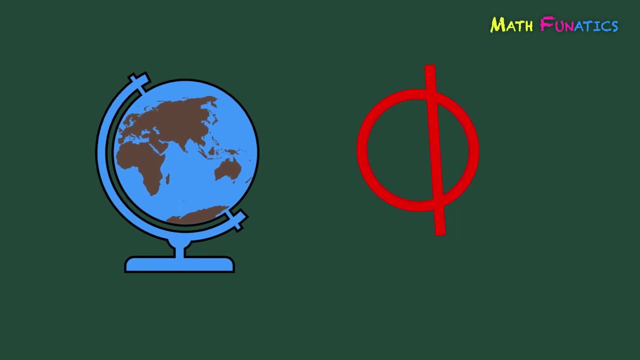 This case, when a line intersects or meets a circle at two points, is called secant. In this situation, the straight line and the circle have two common points or points. In this situation, the straight line and the circle have two common points or points. 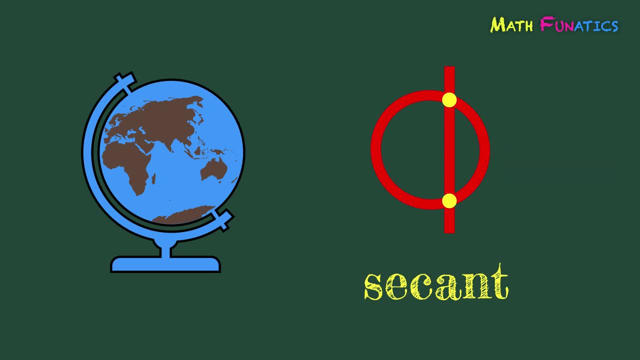 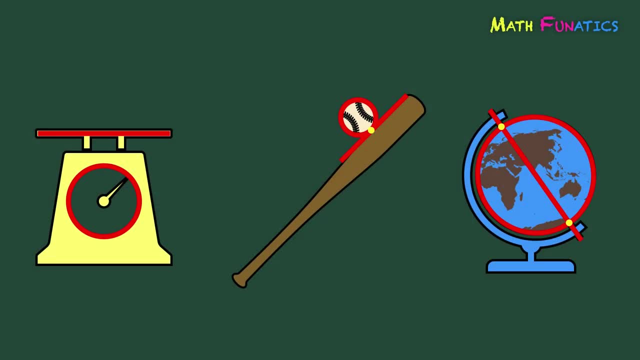 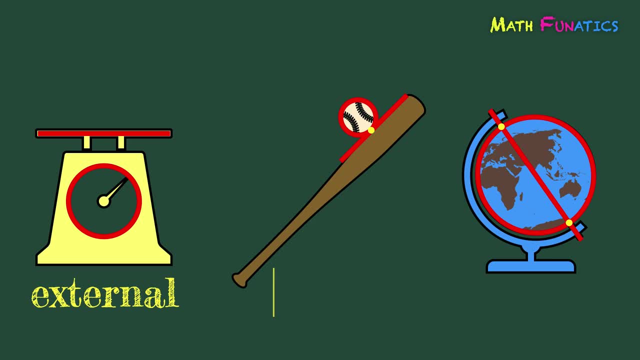 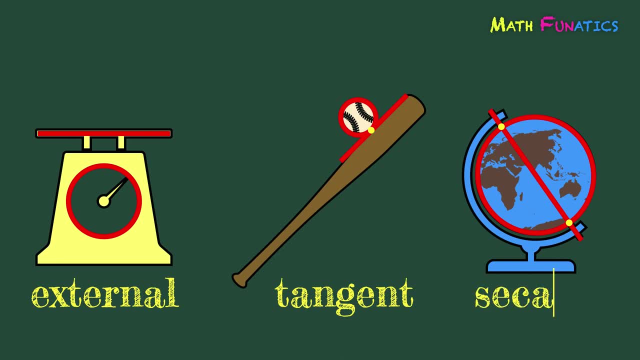 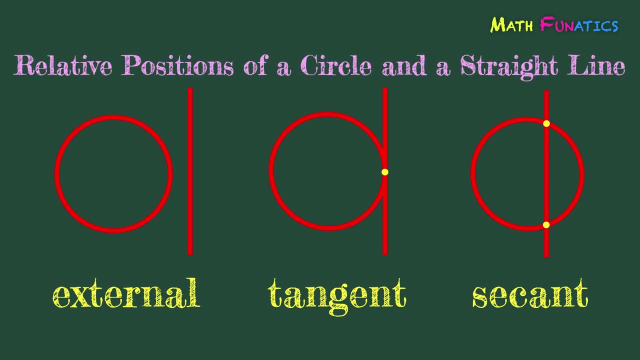 In this situation, the straight line and the circle have two common points or points of intersection. All these three are the relative positions of a circle and a straight line. Again, a straight line having no point in common with a circle is called external. On the other hand, a straight line which meets or intersects the circle at one point is called tangent. 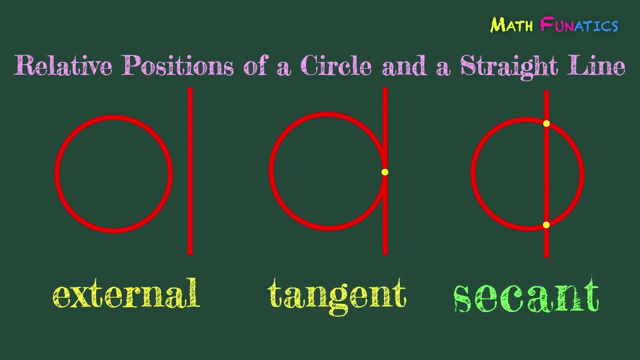 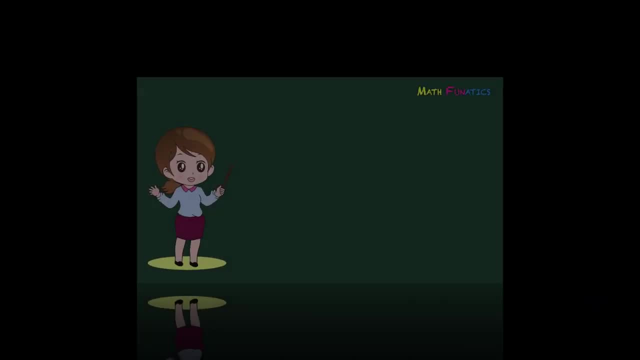 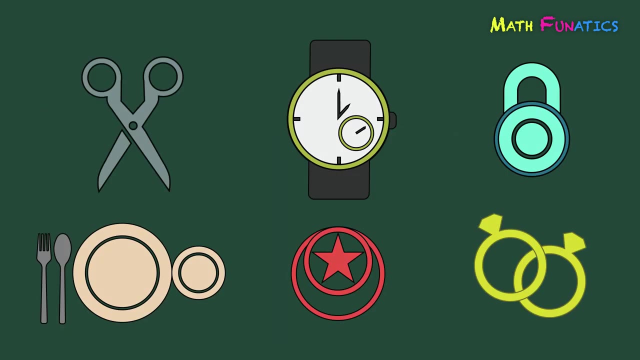 And a straight line which meets or intersects the circle at two points is called secant. This time, let's learn more about relative positions between two circles. Let's take a look at the following illustrations. We have a pair of scissors, A wristwatch, A padlock. 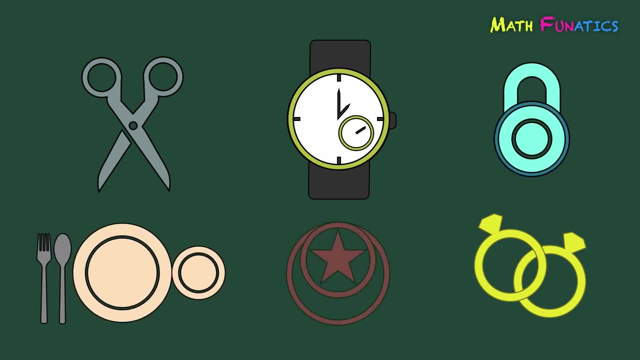 An eating set, A lantern And two rings. Notice that there are circles in each illustration. The pair of scissors has two circular shapes on its handle. The wristwatch has a circular edge and a smaller circle inside it. The body of the padlock is also circular in shape and has a smaller circle in the middle part. 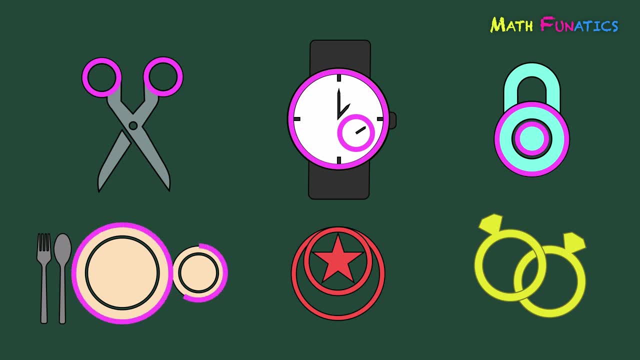 The plate in the eating set. The plate in the eating set is circular in shape and touching its edge is a circular saucer. The lantern has a circular edge and a smaller circle on it, And the two overlapping rings are also circular in shape. Let us analyze each pair of circles in the first three figures. 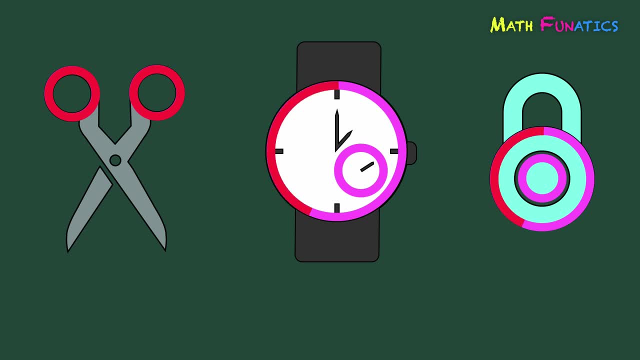 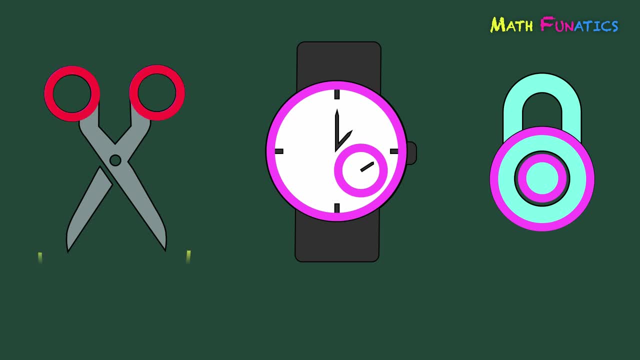 As you've noticed, all these pairs of circles do not meet or touch each other. the pair of scissors are located outside of each other, while on the watch and padlock the smaller circles are located inside the bigger ones. specifically, we use the term external if one. 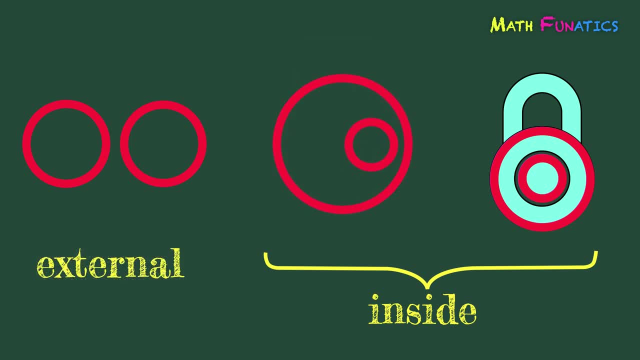 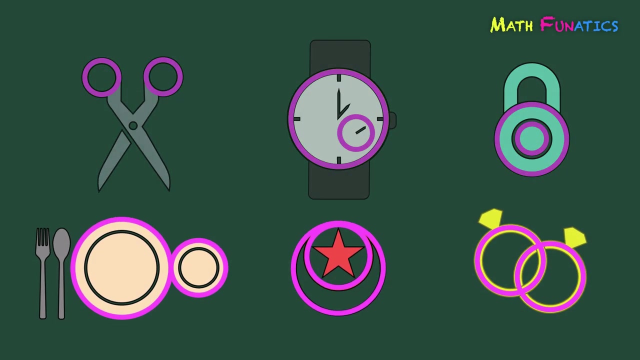 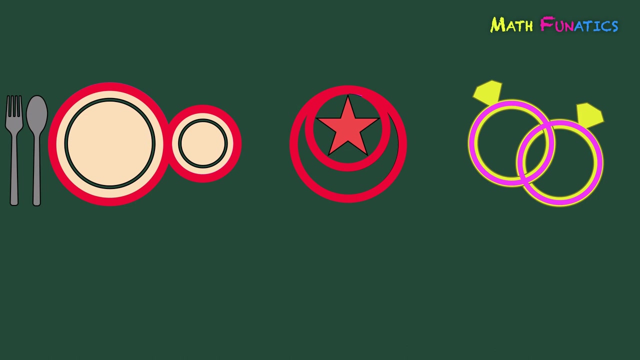 circle is completely outside the other circle, internal if one circle is completely inside the other circle and if the circles share a common center. we use the term concentric this time. let us analyze each pair of circles in the next three figures. as you've noticed, all these pairs of circles do meet or touch each other at certain points. 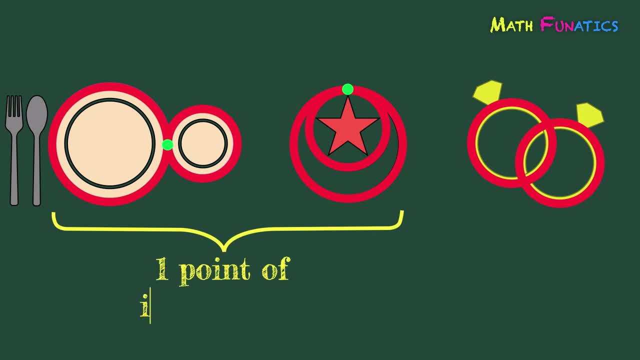 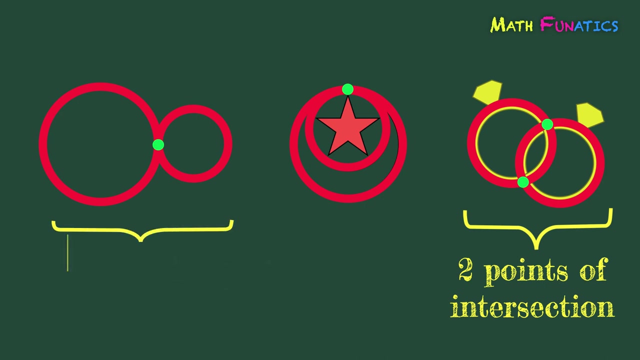 each pair of circles in the eating set and land has one point of intersection, while the two overlapping rings have two points of intersection. if the circles have one point of intersection, then we use the term tangent. if the circles intersect at one point externally, then we call this as externally tangent. 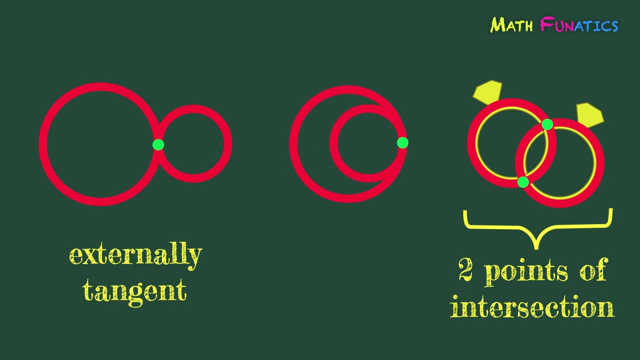 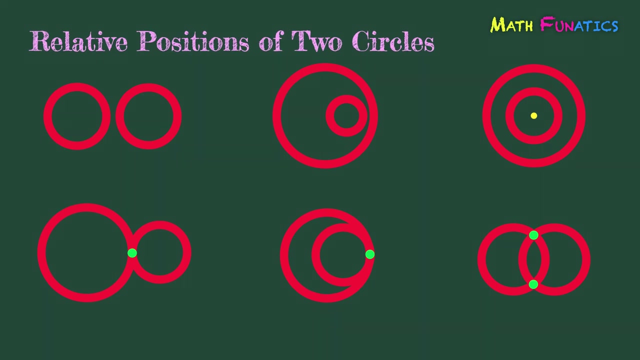 if the circles intersect at one point internally, then we call this as externally tangent, and if the circles intersect or meet at two points, then this is what we call as secant. all these six illustrations are the relative positions of two circles. let's identify each. we have the external, internal, concentric, externally tangent. 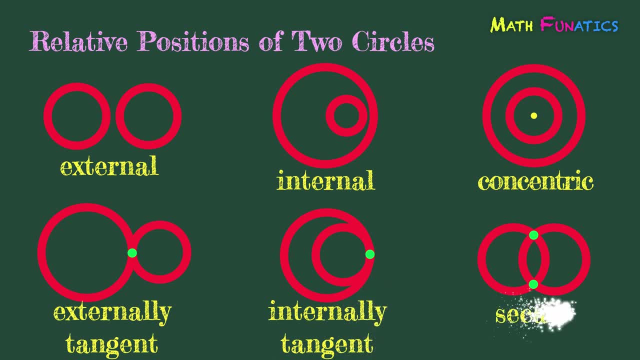 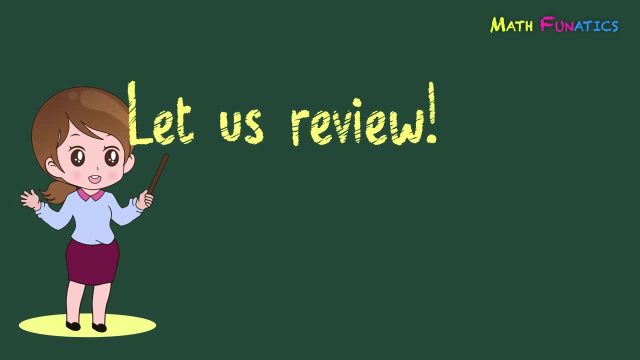 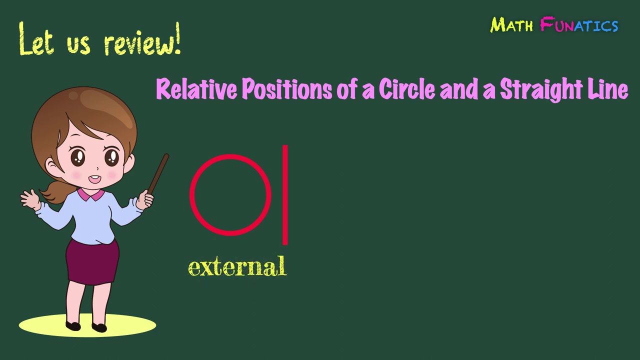 internally tangent and secant. good job, students. now let's make a recap of what you've learned today. there are three relative positions of a circle and a straight line. first, if a straight line has no point in common with a circle, then it is called external. second, if a straight line meets or intersects, the point is called external. if a straight line meets or intersects, the point is called external. and if a straight line meets or intersects, the point is called internal. 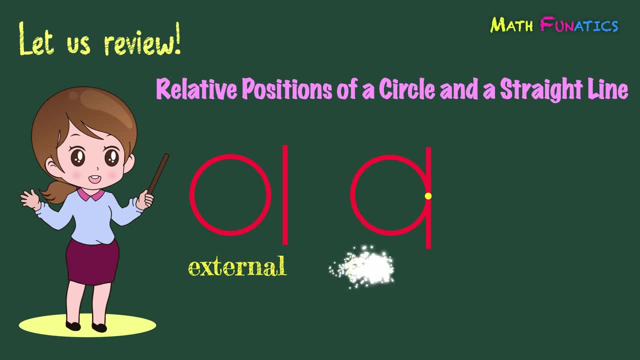 the circle at one point, then it is called tangent. Third, if a straight line meets or intersects the circle at two points, then it is called secant. There are six relative positions of two circles. If one circle is completely outside the other circle, then it is called external. If one circle is